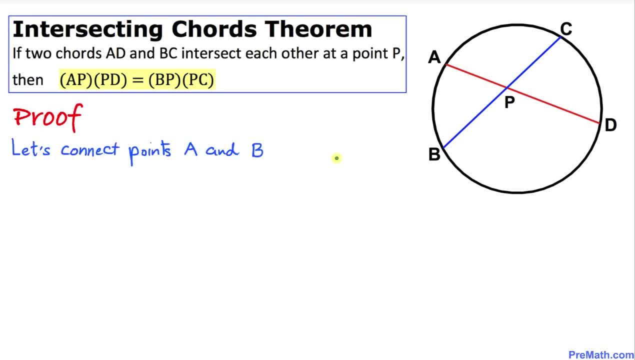 here is our very first step. Let's go ahead and connect points A and B first. Let's go ahead and carefully connect A and B, and we are going to connect points C and D as well. Let's go ahead and connect C and D, And here is our. 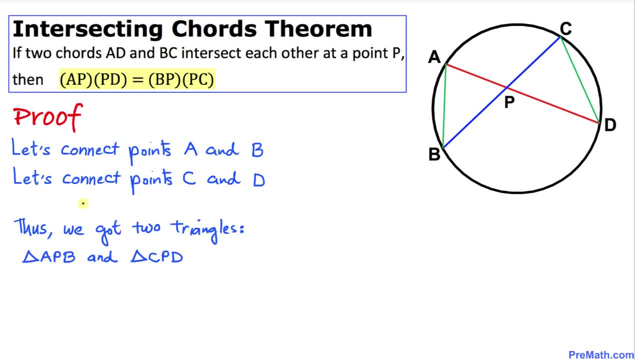 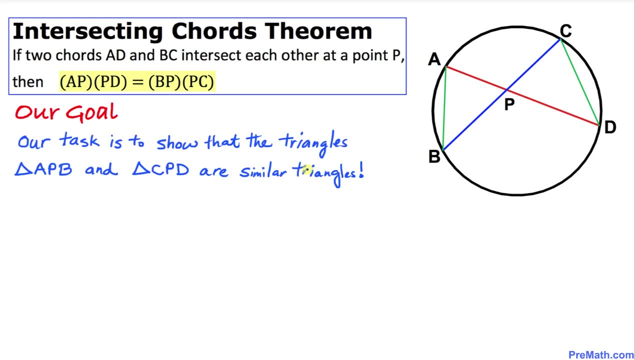 markup, much nicer looking diagram and, as you can see that we got two triangles: one is APB and the other one is triangle CPD, and here is our action plan. we are going to show that these triangles, APB, and the other triangle, CPD, are similar triangles, and here's the beginning of our formal proof. 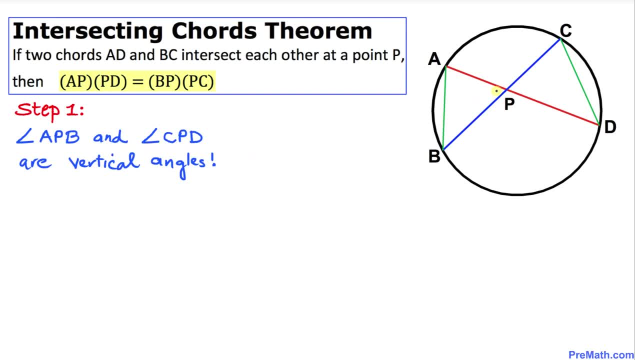 let's focus on these angles: APB, this one and the angle. the other angle is CPD. they are vertical angles and here's the vertical angles theorem. vertical angles are pair of opposite angles formed when two lines intersect. as you can see over here, vertical angles are always equal to each other over. 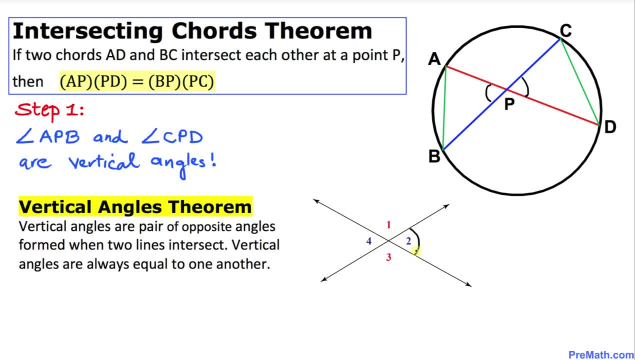 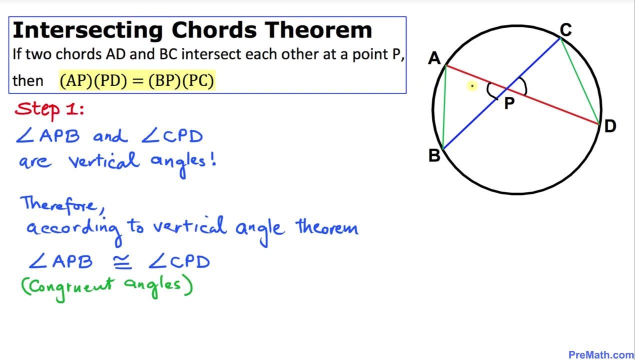 here this: vertical angle 2 and vertical angle 4: they are equal, and the vertical angle this 1 and the vertical angle 3, they are equal as well. so therefore, according to vertical angle theorem, these two angles, APB and CPD, are congruent. and, by the way, 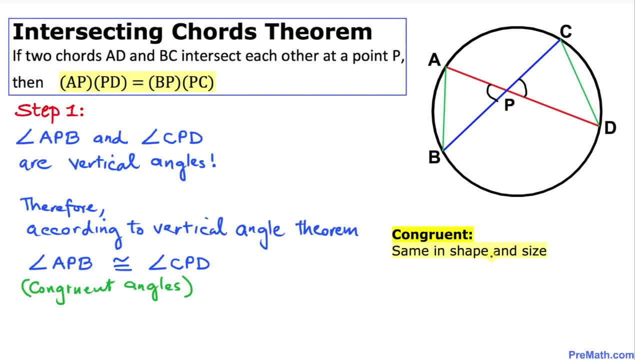 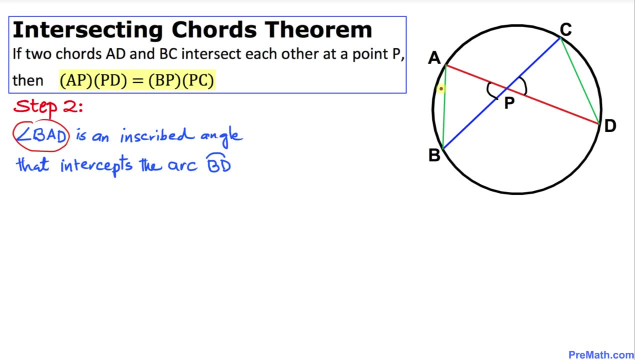 congruent means same in shape and size. and here is our next step. let's focus on this angle BAD, this angle BAD. this is an inscribed angle that intercepts the arc. we can see arc BD. and here's the inscribed angle theorem, the measure of 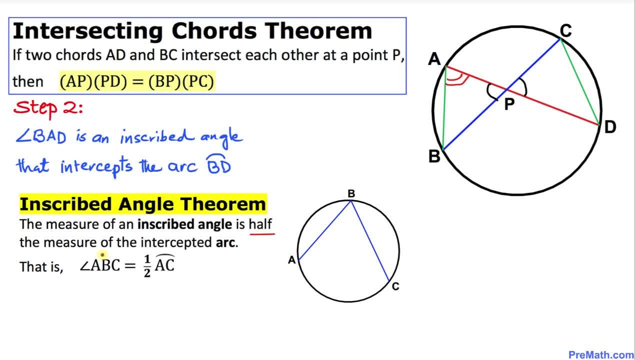 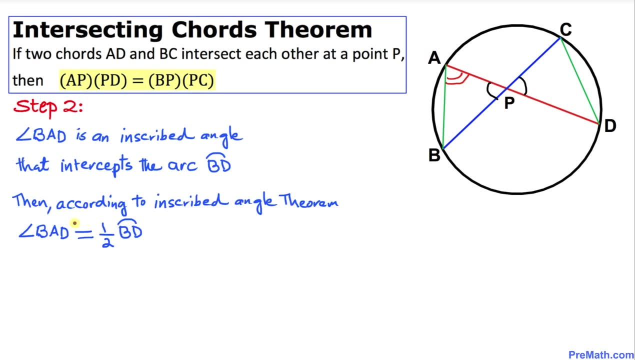 an inscribed angle is half the measure of the intercepted arc, that is, this angle ABAD C is equal to the half of this arc, AC. so thus, according to inscribed angle theorem, this, our angle BAD, equals to the half of this intercepted arc, BD. and I'm 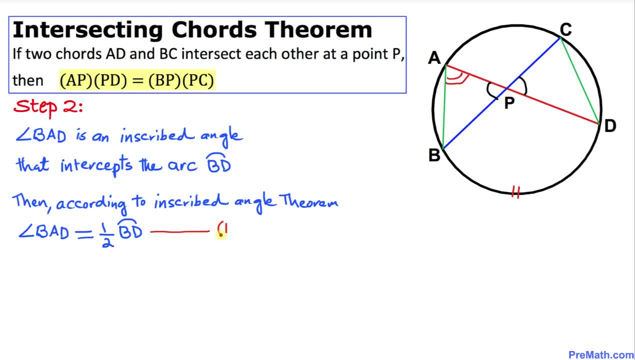 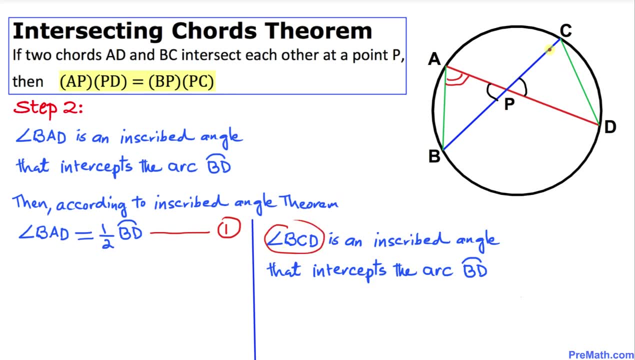 going to call this one as an equation number one. and now let's focus on this angle BAD. and now let's focus on this angle. BAD. and now let's focus on this angle BAD. and now let's focus on this angle BCD. right over here. it is also an 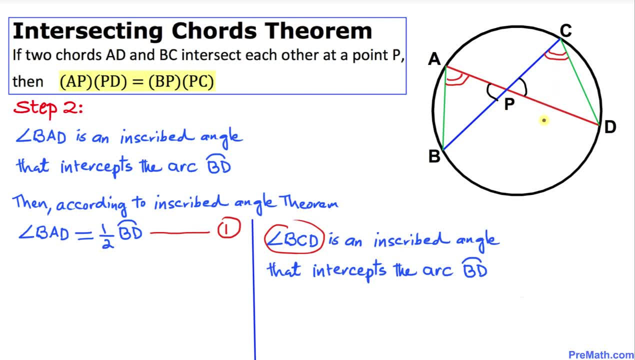 angle BCD right over here. it is also an angle BCD right over here. it is also an inscribed angle that intercepts this arc inscribed angle that intercepts this arc inscribed angle that intercepts this arc BD. so therefore, according to the very 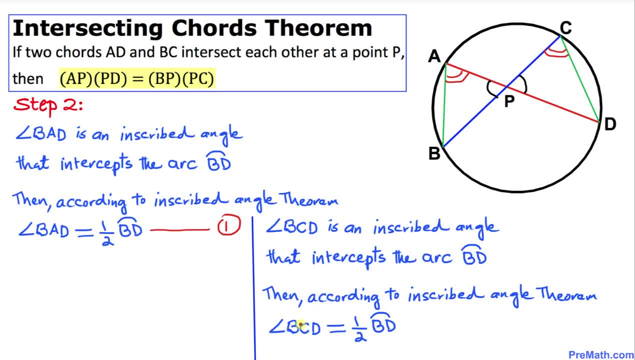 BD. so, therefore, according to the very BD. so therefore, according to the very same inscribed angle theorem, this angle, same inscribed angle theorem, this angle, same inscribed angle theorem, this angle, BCD equals to a half times this. BCD equals to a half times this. 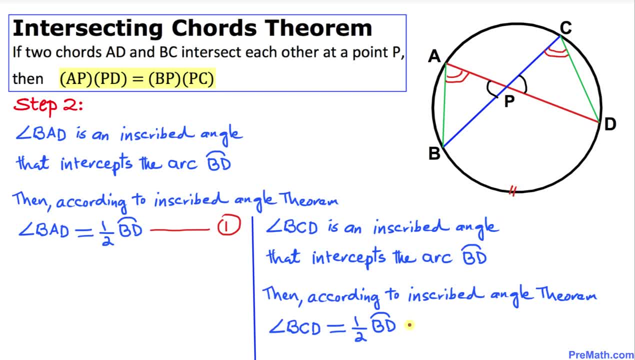 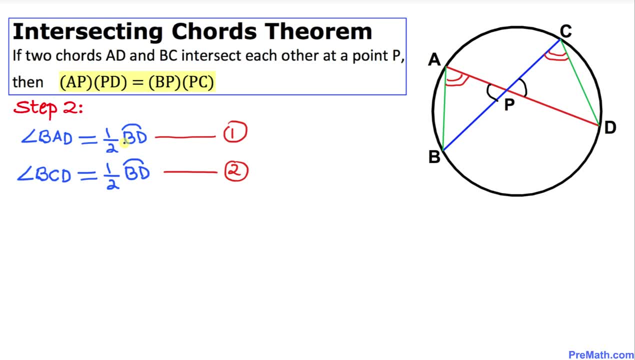 intercepted arc, which is bd, and i'm going to call this as an equation number two, and here i have wrote down these two equations separately. let's go ahead and compare these two equations, as we can see that the right hand side of these two equations are same, so that means we conclude that the left 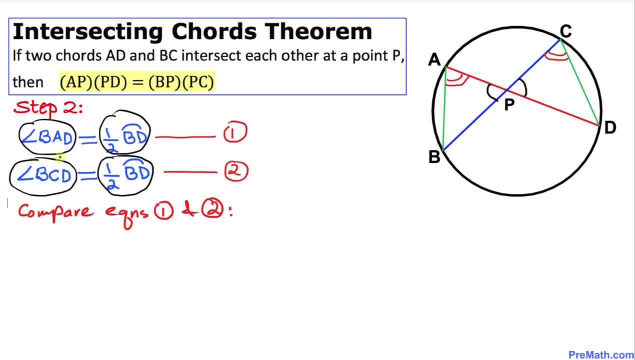 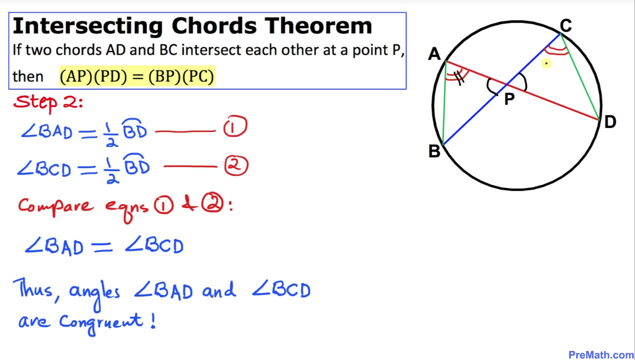 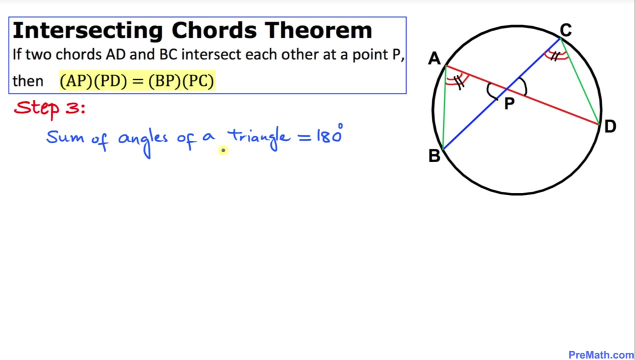 hand side are equal as well. so therefore, this angle bad turns out to be equal to angle bcd. so that means these two angles bad and this angle bcd are congruent, and we know that the sum of the angles of a triangle is always 180 degrees. 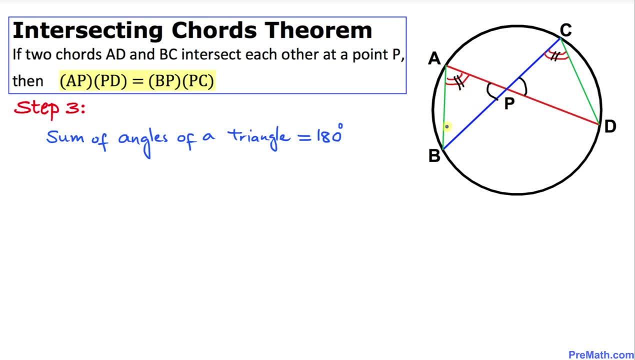 and we know that the sum of the angles of a triangle is always 180 degrees, and we know that, And if we can focus on these two triangles, this third angle, then, is going to be congruent to this angle. all right, Because now the sum of these three angles is going to be 180 degrees and likewise, this is going to be 180 degrees as well.